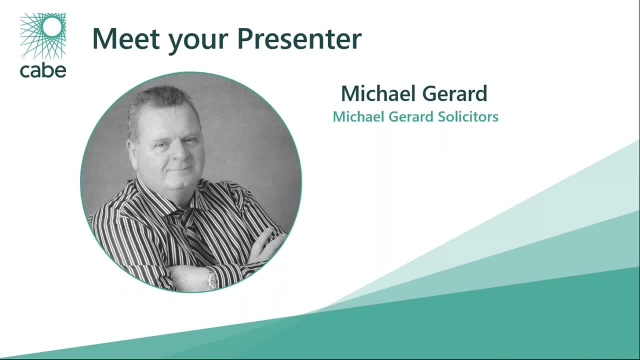 in adjudication proceedings and ADR. Clients include principal and specialist contractors, industry professionals, local authorities, developers and employers. Michael's experience includes a range of public and private sector projects, from schools, hospitals and housing to military and nuclear installations. He has also been involved in numerous instructions. 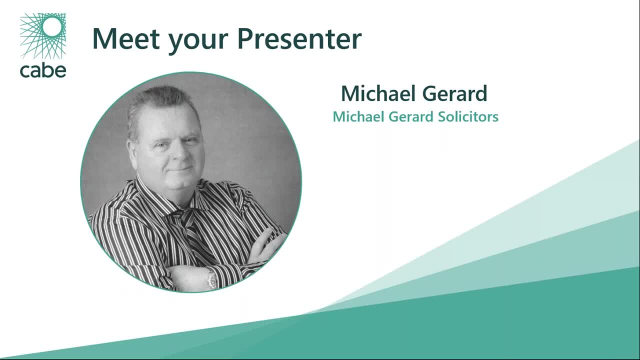 relating to tribunals and court proceedings. Michael has also been involved in the formation of the National General Audit and the National Commission for Regulatory Policy for the case management, as well as in excess of 100 adjudications as adjudicator and party representative. Michael regularly has articles published in the media and also lectures on various 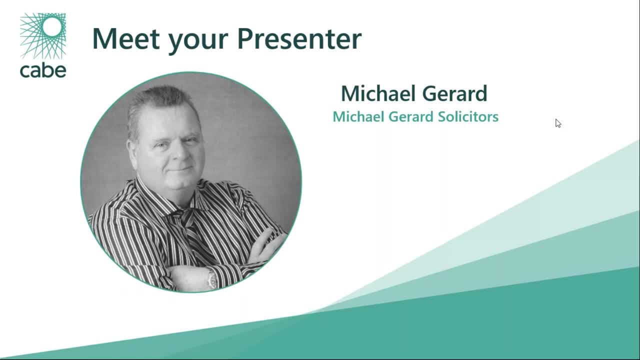 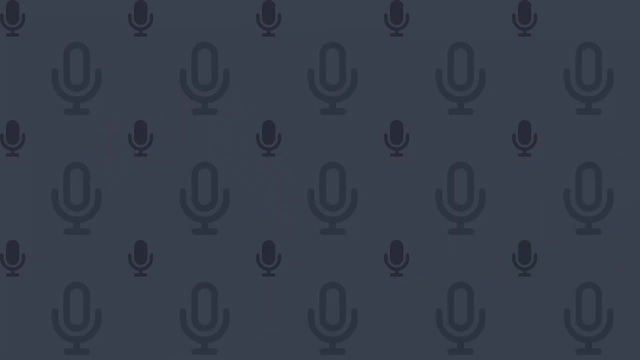 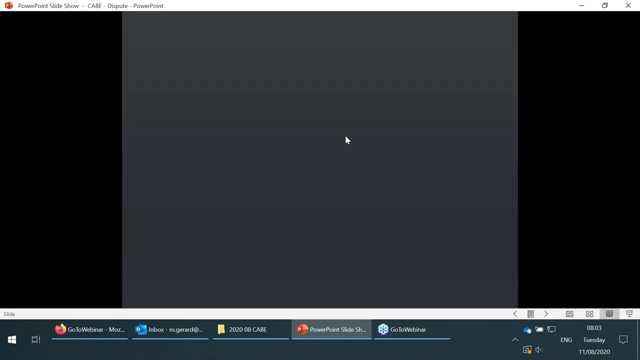 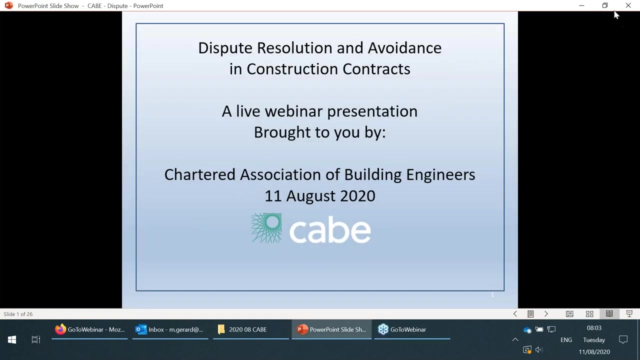 aspects of construction law. and with that, in a couple of seconds, I will hand over to Michael and he can go through the session with you. Michael, Good morning. thank you for that introduction. uh, Jordan, much appreciated. and that cuts out instantly the first couple of slides I've actually got up here. 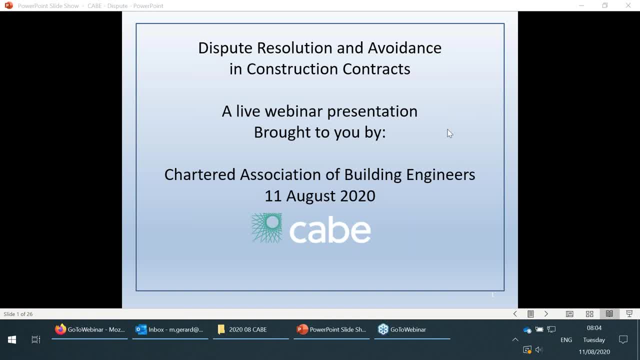 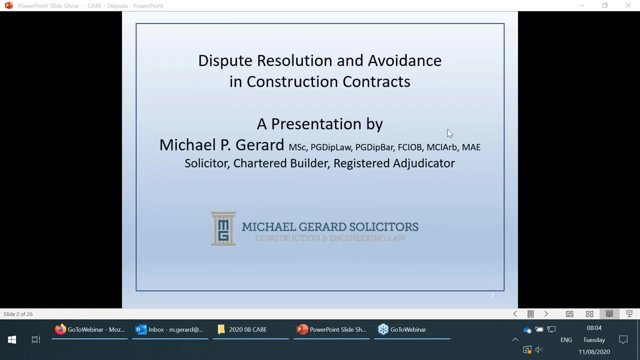 as, yes, this is a live webinar presentation brought to you by the Charleston Association of Builders, нас triage engineers, and I do thank CABE for allowing me to actually present this to this presentation to you all this morning. as Jordan was saying, I am Michael Gerrard, I'm a practicing solicitor, charter builder and registered 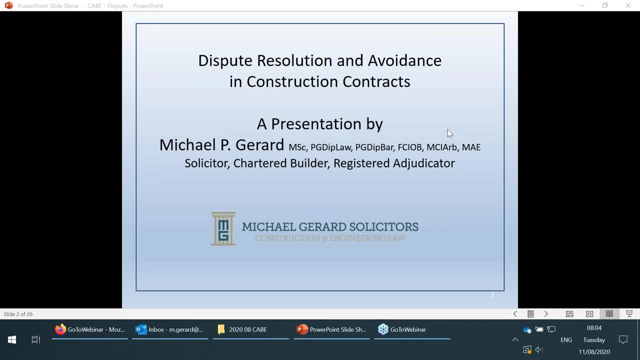 adjudicator, and my presentation this morning is on dispute resolution and avoidance in construction contracts. this is aimed for those that have very little experience in this area, and so I do apologize for those that's also attending this if your level is slightly above this, but I think it's it does that. 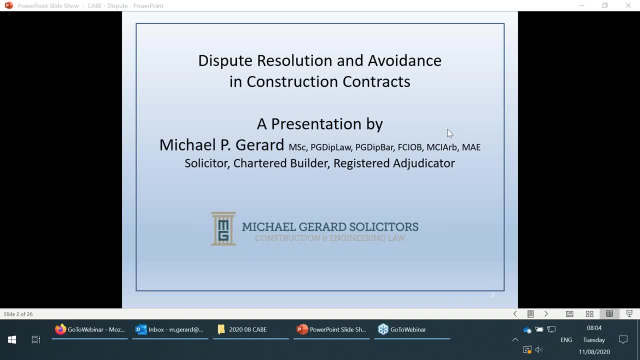 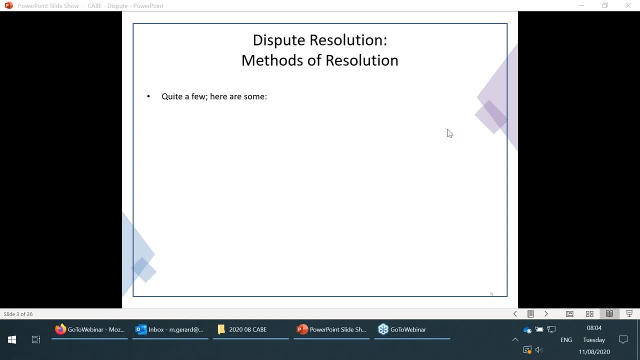 there's a lot of demands for this in relation to the the issue that that we actually are working without further ado, a district resolution. methods of resolution: there are quite a few. we have you litigation, arbitration, negotiation, mediation and conciliation, adjudication, expert determination, mini trial, dispute boards, and of those methods of resolution, 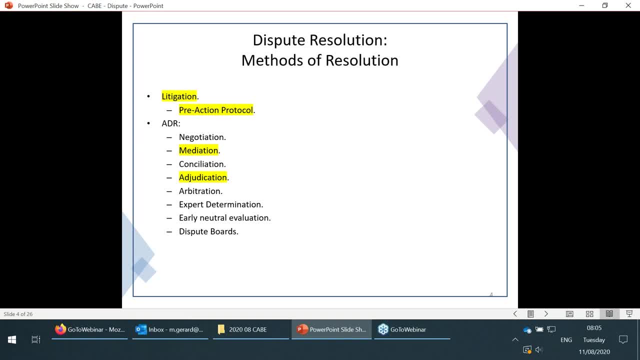 they can be divided up into two categories. you've got litigation, which is a standalone form of method of resolution, and then basically anything else which is not litigation can be put under the umbrella of ADR, alternative dispute resolution. now I have that. the ones I've highlighted here are the ones 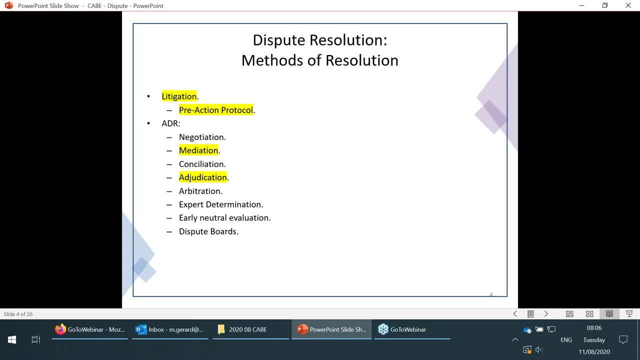 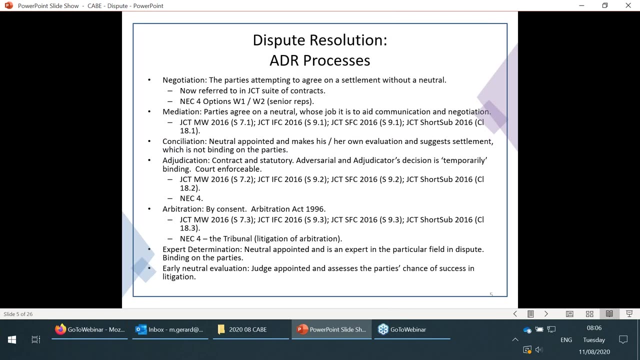 that I'm going to be speaking about in more detail in this presentation, because these are the ones that is most commonly used within the construction and engineering industries. ADR processes: we have negotiation. they, very briefly, this is: this is where the parties attempt to agree on the settlements without a neutral. essentially, 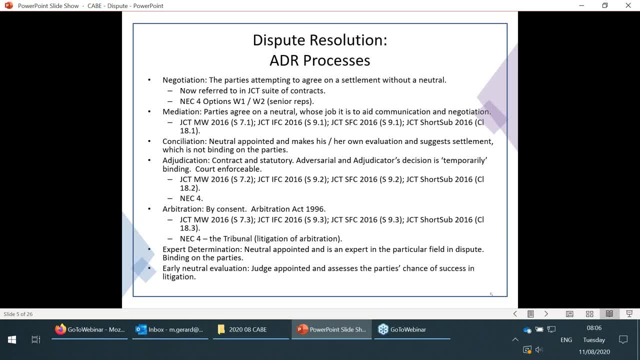 it is the two parties that have a dispute that essentially get around a table without any party representative. this is also now referred into the JCT suit of contracts and it's all also referred to in the NEC for w1, w2 very, very roughly. it's in relation to the senior representatives of a company that 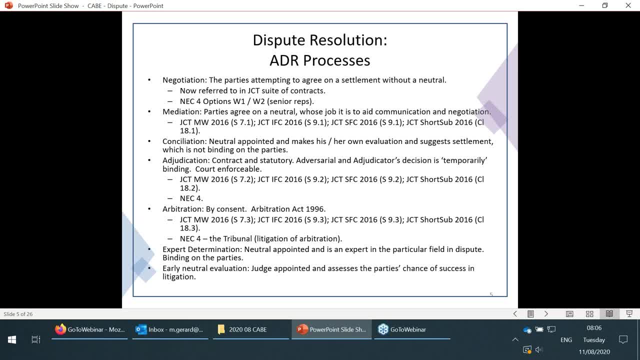 actually gets given so that she lumps then under negotiation mediation. this is where the parties agree on a third party, a neutral third party whose job it is to aid communication and negotiation, and again, this is referred to in all the the current JCT suites of contract consideration. 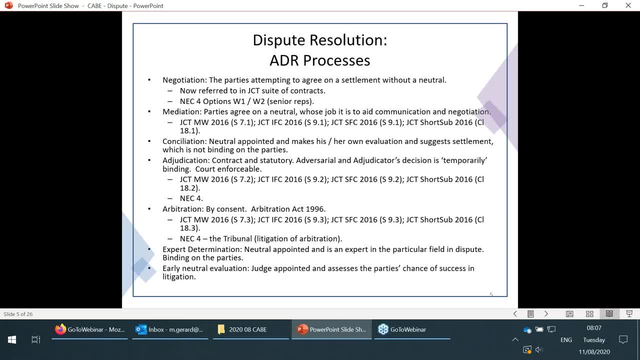 this is where a neutral is appointed and makes his or her own evaluation and suggests settlement that it's not binding on the parties, unless, of course, the parties enter into a settlement agreement. adjudication: all of you should be familiar with adjudication, albeit not in the detail, but we have essentially two types of adjudication: contract and statutory. this 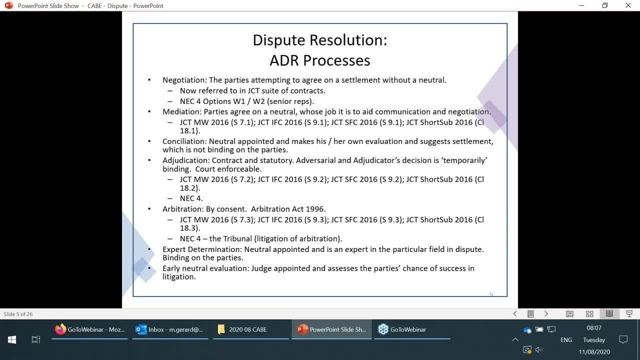 is adversarial and the adjudicators decision, once published, is temporarily binding and, of course, is caught enforceable. this is referred to in again all the JCT suites of contracts and other standard forms of contracts, including the NEC arbitration. this is by consent and it's governed by the Arbitration. 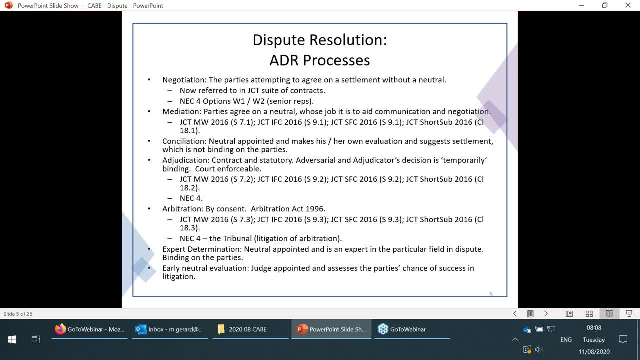 Act 1996 in this country and again the JCT and the NEC refers to this. although the NEC refers to a tribunal, which is either litigation or arbitration, expert determination is where a neutral is appointed and that neutral is an expert in her or his particular field in relation to the dispute and it's binding on the parties. 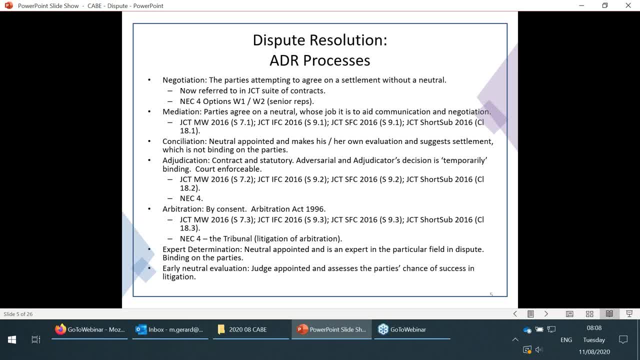 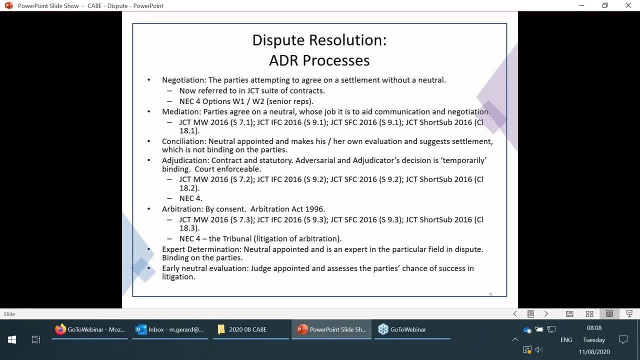 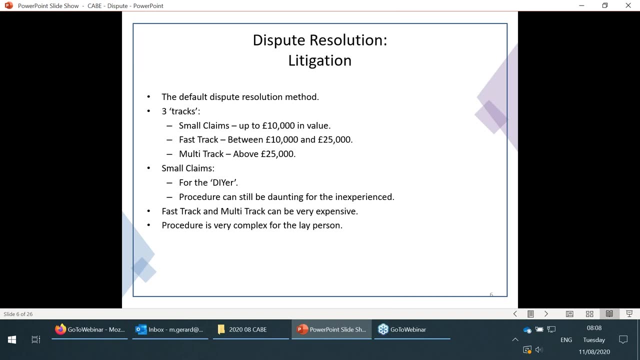 and early neutral evaluation is where a judge is appointed and assesses the party's chance of success in litigation. litigation: this is the what I would refer to as a default dispute resolution methods. certainly because anyone can actually refer to the dispute resolution method as a default dispute resolution method. certainly because anyone can actually refer 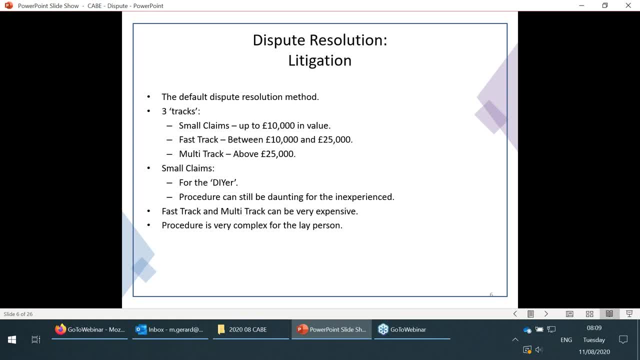 a matter to litigation, especially where there is no mention of the form of dispute resolution within the contract and under litigation. there are three tracks. you have the small claims track, which is anything up to £10,000 in value. you have the fast track and that is. 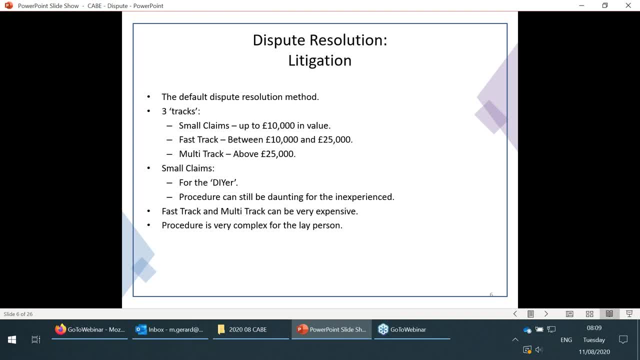 any disputes with a value between £10,000 and £25,000, and the third track is called the multi-track, and this is above £20,000.. Small claims, as you would no doubt guess, is for the DIYer, although the procedures can still be daunting for the inexperienced, and the fast track and multi-track can be very 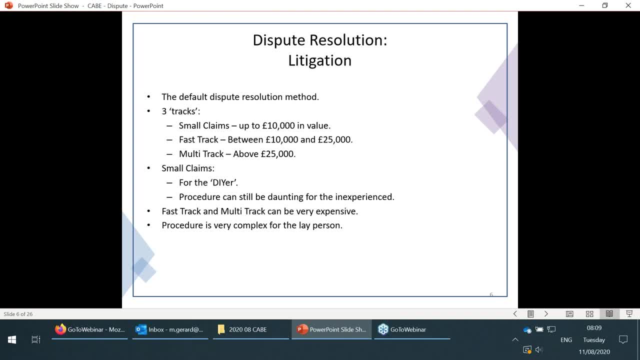 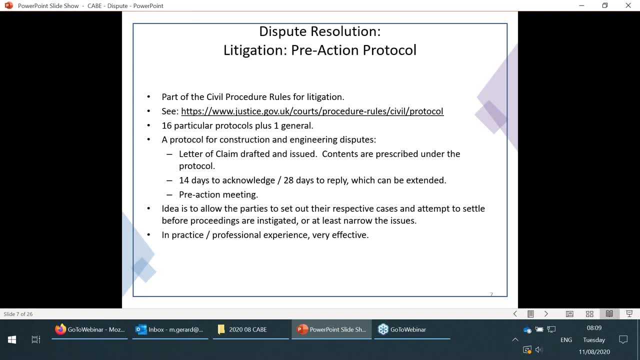 expensive and for all of the tracks the procedure is quite complex for lay people. In litigation, you also have what you call the pre-action process protocol and this is part of the civil procedure rules for litigation. now, on an earlier slide, where I highlighted the forms of dispute resolution, I also highlighted pre-action protocol under 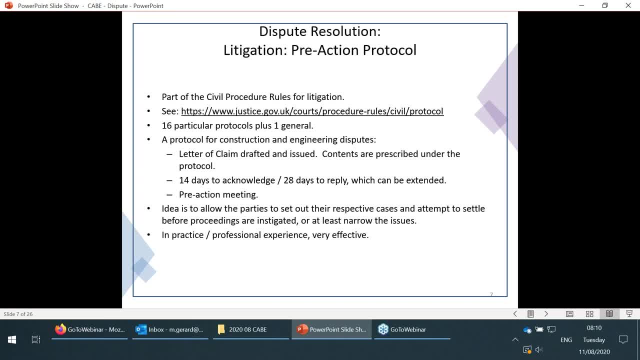 litigation. although it is part of litigation, it is also a quite an independent form of dispute resolution in itself. there are 16 particular protocols plus one general. one of the particular protocols is for construction and enduring disputes and essentially the pre-action protocol is all but mandatory for those that's entering into a disputes resolution. 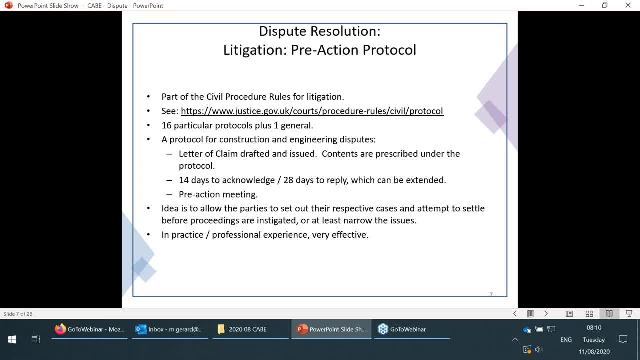 that involves litigation. and these procedures, or the the pre-action political, must be instigated before you run off and issue proceedings. and what happens under the pre-action protocol is that a letter of claim is drafted and issued by the claiming party. the contents of that letter, of that letter of claim, is prescribed under the pre-action protocol: the 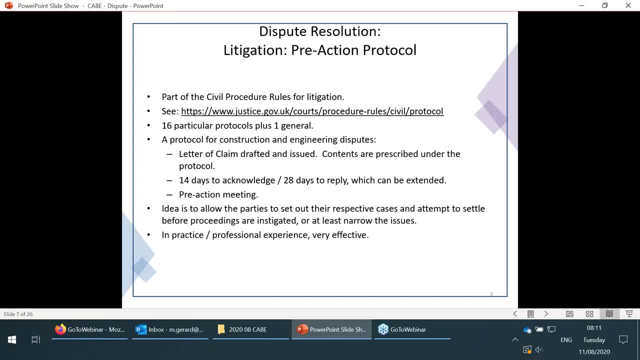 the other side of the defending party has 14 days to acknowledge and 28 days to reply, and and also a counterclaim can also be included as well. this can be extended. quite often it is extended and then, once the parties have exchanged their their statements, a pre-action meeting is. 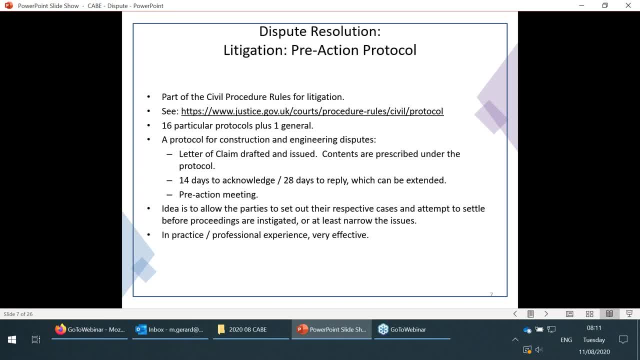 usually called. now, very often we have mediation and in mediation, essentially my experience under the pre-action protocol is very, very successful and the idea of a pre-action protocol is to allow the parties to set out their respective cases in an attempt to settle before proceedings or instigated or, at the very least, narrow the 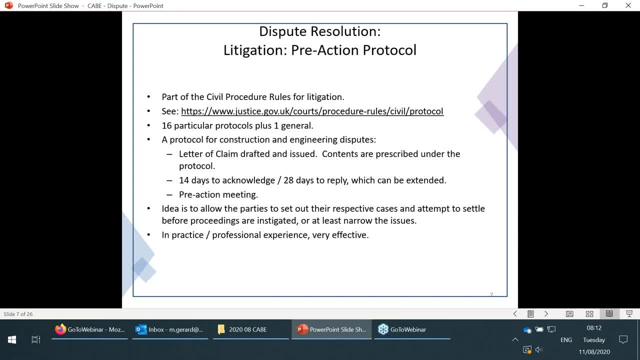 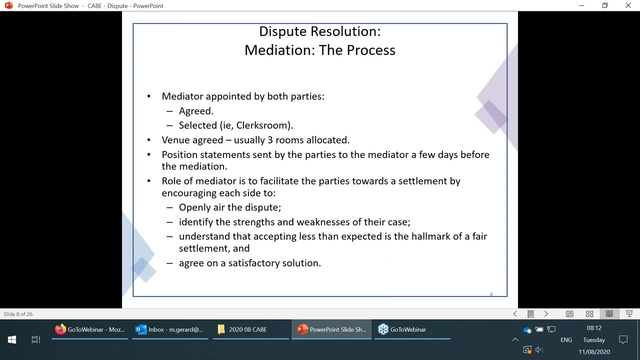 issues. this is because we're trying to cut down on costs, which is very, very costly to run off and and litigate the the actual, the actual dispute and, as I said before, is that in practice, in my professional experience, this is very, very effective. stage mediation, the process, a mediator. 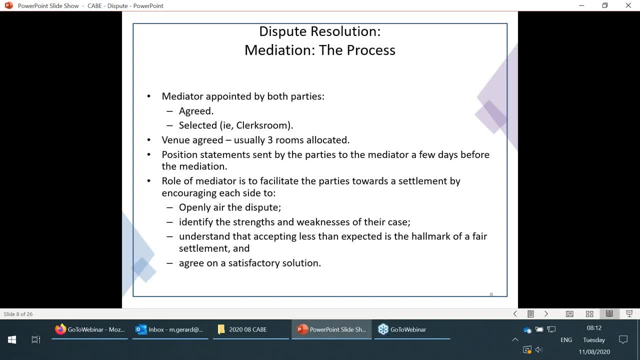 is appointed by both parties. the mediator can be agreed by both parties or you can go to a recognized um mediation organization that will select a mediator or at least put forwards, uh, three mediators that fit within the, the area expert expertise that you actually require um the. the venue is agreed by the parties. usually there's three rooms allocated, that is for 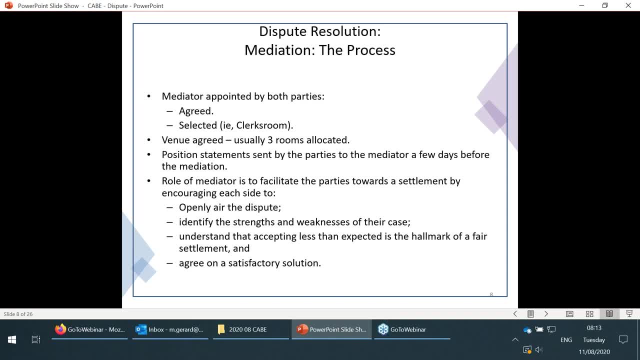 um, both parties will have their own rooms and you will have a central a room where the parties uh come together um now and again throughout the uh, the uh, the mediation process, and also, of course, mediator, and can actually uh sit as well before the uh, before the media, the actual mediation. 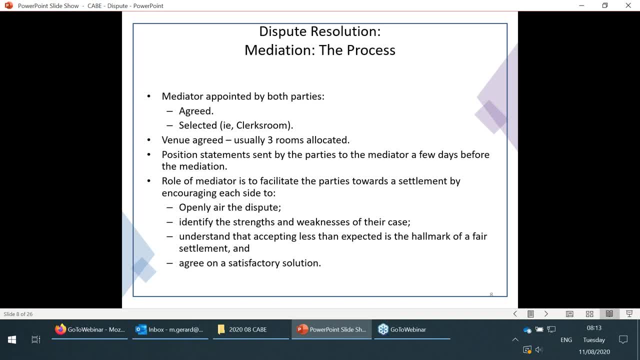 parties will exchange statements and they will be sent to the mediator just a few days before the mediation to give the mediator a very good understanding of what the district is about. and the role of the mediator is to facilitate the parties towards a settlement or encouraging each side to openly air the dispute, identify the strengths or weaknesses of their case. 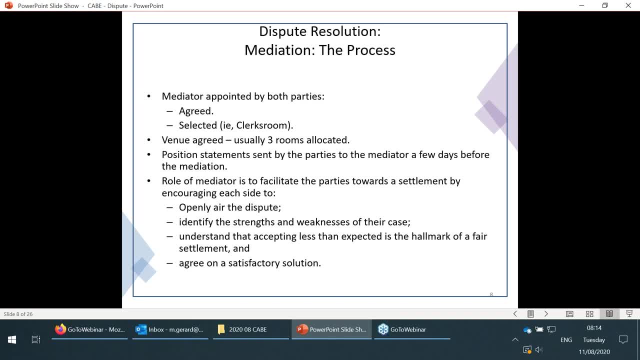 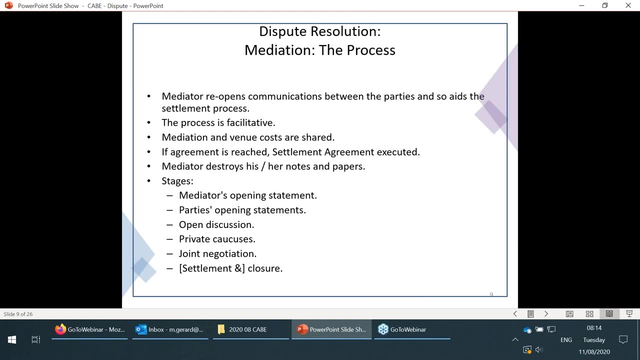 understand and accept. accepting less than expected- expected is a hallmark of a fair settlement and to agree on a satisfactory conclusion, the mediator reopens communication between the parties and so aids the settlement and the process is facilitates the actual- uh, the actual, the actual process that the mediator will not give an opinion. 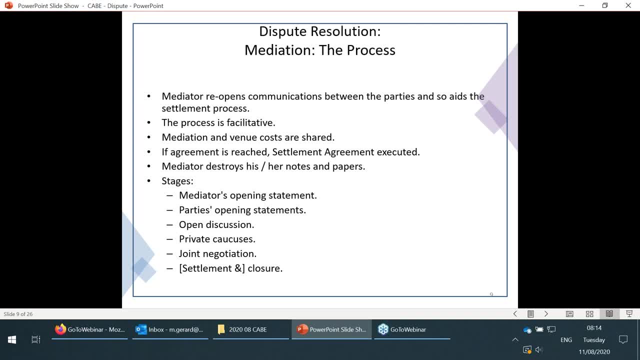 but what will happen is that when the parties are in their separate rooms, the mediator will actually dart between the two rooms um listening to to the parties, taking communication straight messages from the other party into to the other party, providing obviously he or she has got published this to the 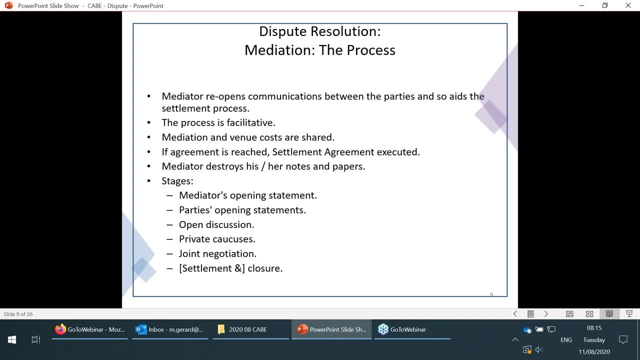 is over, whether it's been settled or not, the mediator will destroy his or her notes and papers. so to recap, you have the mediators opening statements, you have the parties opening statements. you have then have an open discussion. you then have the fallouts in relation to both parties going off into their own. 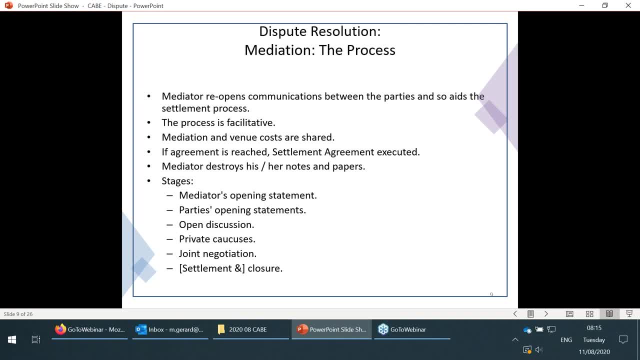 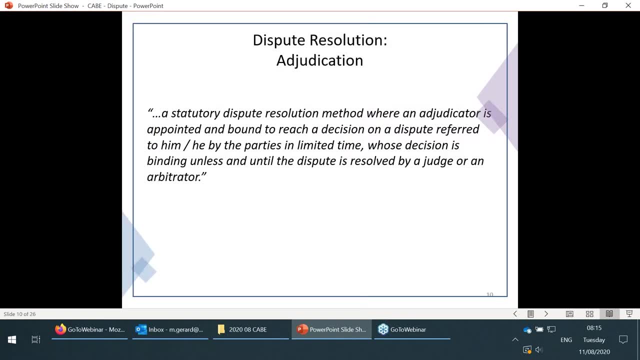 rooms. then you'll have the joint negotiation and hopefully at the end of that process you'll have settlements and closure adjudication. I quote a saturated dispute resolution methods where the adjudicator is appointed and bound to reach a decision or the disputes refer to him or her by the 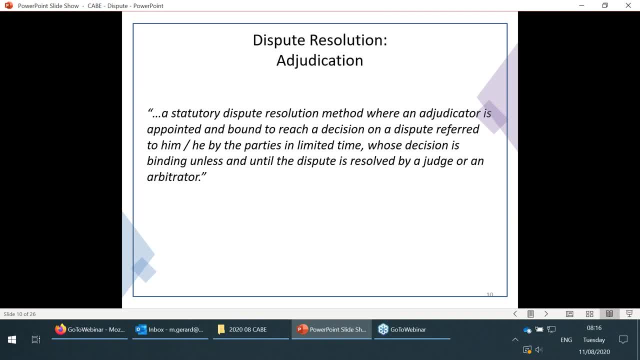 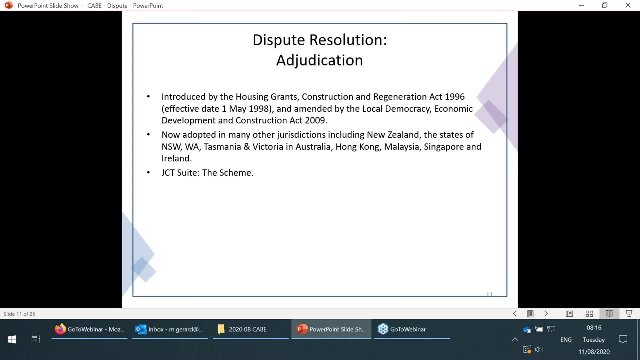 parties in limited time, where the decision is binding unless and until the disputes is resolved by a judge or an arbitrator. this adjudication was introduced by the housing grants construction Regeneration Act 1996 that became effective the first of May 1998 and it was subsequently. 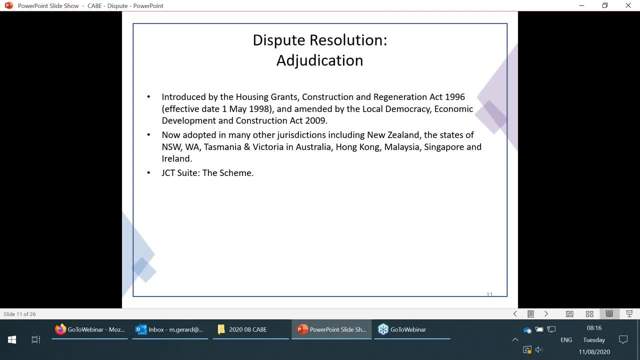 amended by the local democracy, economic development and construction acts 2000 and I think that became effective in- I think it was October 2011.. The adjudication has been so successful here in the UK in relation to structural engineering disputes that many other jurisdictions throughout the world has now adopted adjudication based on what we 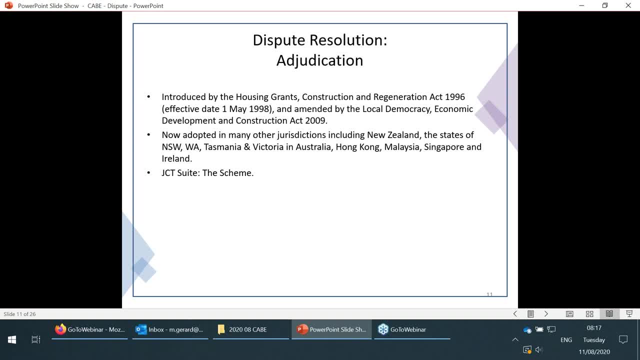 have here, including New Zealand, various states of Australia, Hong Kong, Malaysia and Singapore, The JCT suites. that refers to the scheme, which is the rules. Section 108 of the Construction Act is the right to refer disputes to adjudication Now, even if a contract remains silent on adjudication. 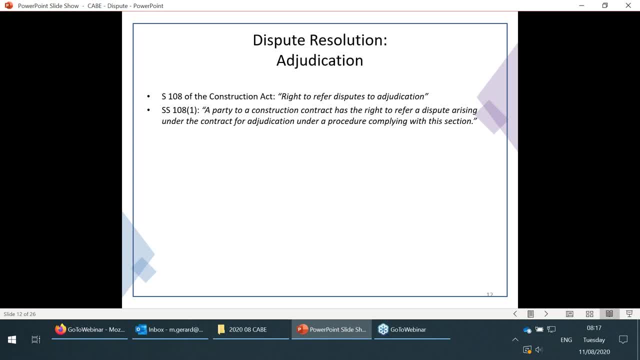 the party still has an absolute right to do so. So a right to refer that a dispute to adjudication, because that is implied by the Act and you can't contract out of the Act. Section 108 subsection 1 is parties to construction contract has a right to refer dispute arising under the contract for adjudication under procedure. 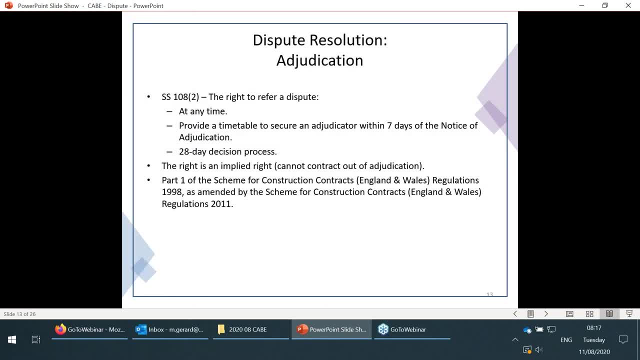 of compliance with this section, Exactly what I've just summarized on that. Section 108, subsection 2, is where you have the rights to refer disputes, which is a right to refer dispute at any time via the timetable to secure an adjudicator within seven days of the notice. 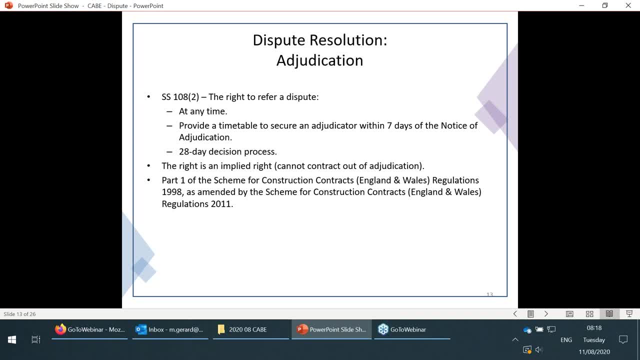 of adjudication. that is very important. the notice of adjudication will actually give a background to the dispute and also it will also have the question or the questions which the adjudicator needs to answer. that is initially served on the referring the responding party and then it then goes off to the AMB which nominates the adjudicator. it's a 28-day decision. 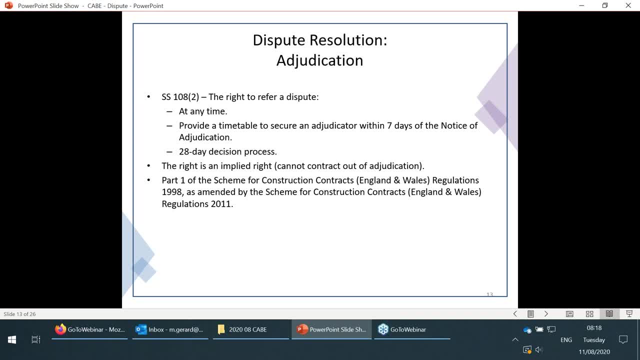 process. so the 28 days will run when the referral notice is issued to the adjudicator. the rights: as I said before, the adjudicator needs to answer the question or the questions which the adjudicator needs to answer the question or the questions which the adjudicator needs to answer the question or the questions which: 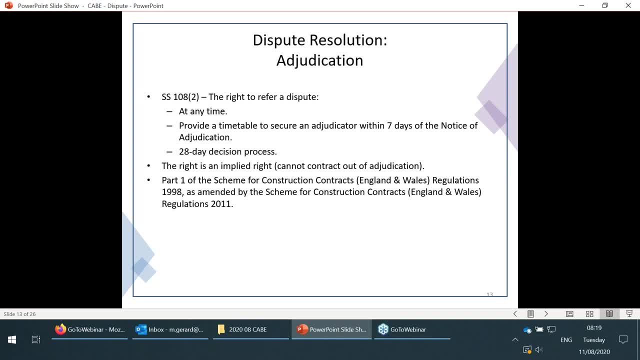 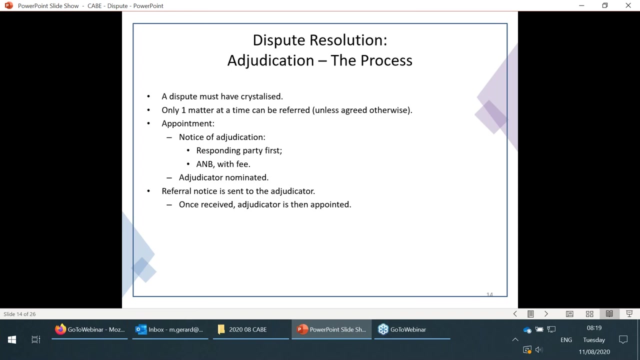 is an implied right in part 1 of the scheme of construction contracts, that is, the rules for adjudication, which, as my last slide had stated, the various standard forms of contract, including the jct, adopts the process first and foremost. you might have already have been familiar with the word. 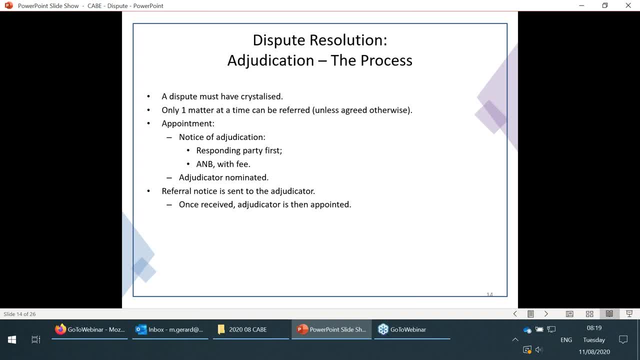 crystallized. that does come out of a the case many, many years ago. please don't ask me about that case because i can't quite remember it, but it is a well-worn word- um and a dispute must have crystallized um district can crystallize uh. 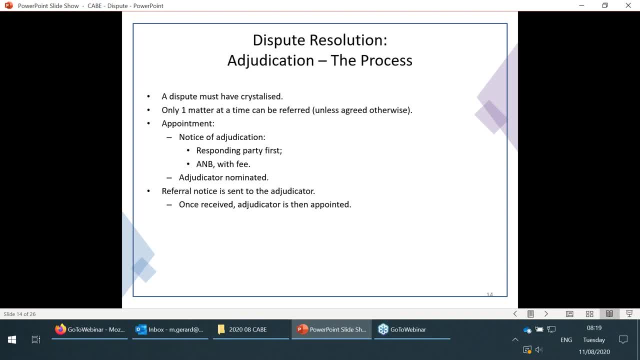 in uh, in many ways. uh, you can even uh, obviously, that the most um, the the most uh. easier example will be where somebody puts uh in a demand for payments, um, or an application and uh, that application, uh, the other side comes back and says, no, i disagree with it. 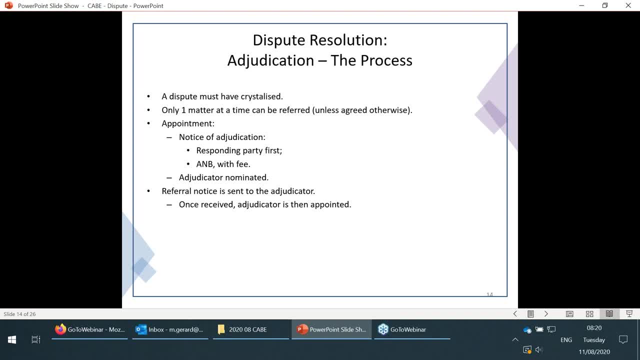 that's a dispute that's crystallized, off you go. it'll also be other areas of uh where even the other party remains silent for a length of time. that could be said a dispute has crystallized because of the silence over that period of time. only one matter. 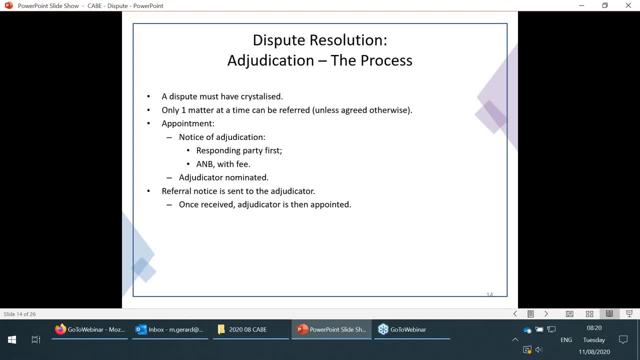 at a time can be referred unless both parties agree that the adjudicator has jurisdiction to decide on more than one dispute. the appointment is, uh, on the notice of adjudication. as i said before, the signing party receives that notice of adjudication. first, very important, and then 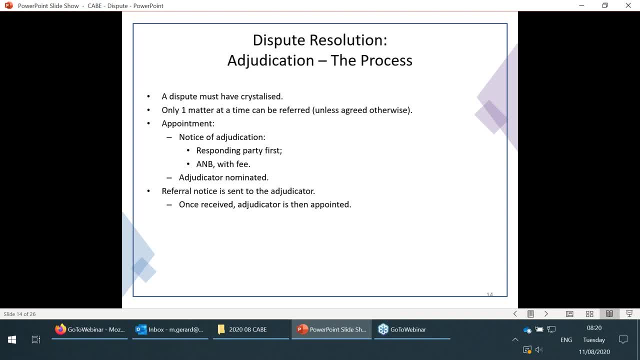 the uh, the body that's going to be nominating the adjudicator- is then issued with the notice of adjudication, along with the application and a small fee- three, four hundred pounds plus the vat- and then the amb will will nominate the adjudicator. the referral notice is then sent to the adjudicator once the adjudicator has been. 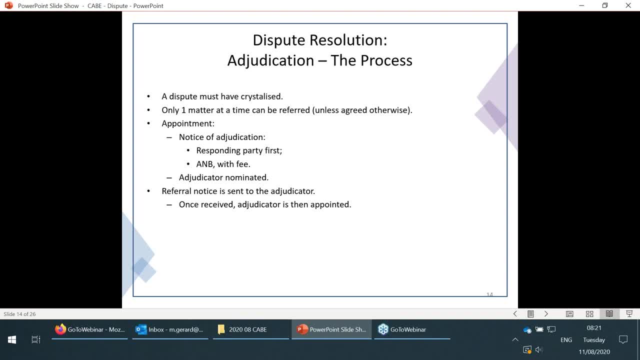 nominated, and once the adjudicator has received the referral notice, the adjudicator is then said to have been appointed. at that point, the adjudicator will then set out his timetable or her timetable, um, and typical information on that timetable will be the date for a possible meeting, the dates, of course, when. 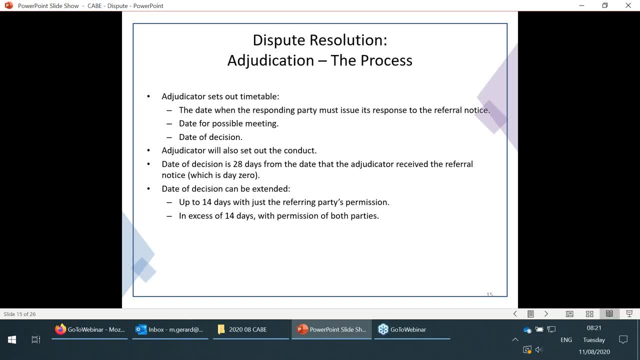 the responding party must issue its response to the referral notice. uh, this can be, most adjudicators will be between seven and ten days and, of course, uh, the dates for the decision that must, must, must make, and that date of the decision is calculated, uh, from the dates that the adjudicator 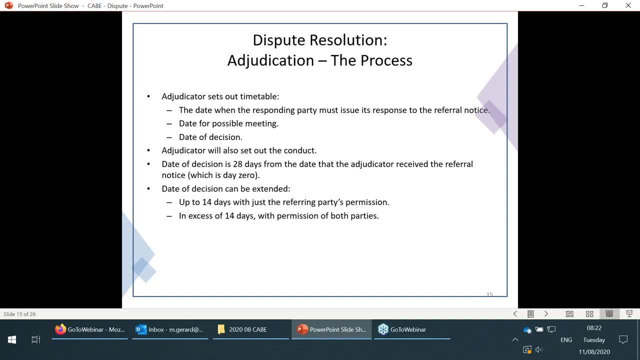 received the uh, the referral notice, plus 28 days, plus uh if there's any bank holidays would also be taken into account as well. the adjudicator also sets out the conduct of the adjudication process, um and um, the uh and the dates of this of the decision. i've said 28 days, but this can be extended. this can be extended by: 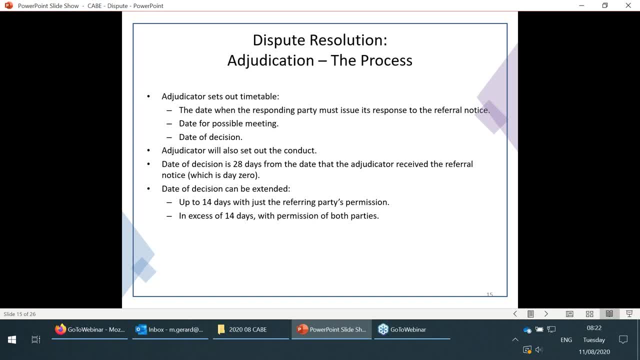 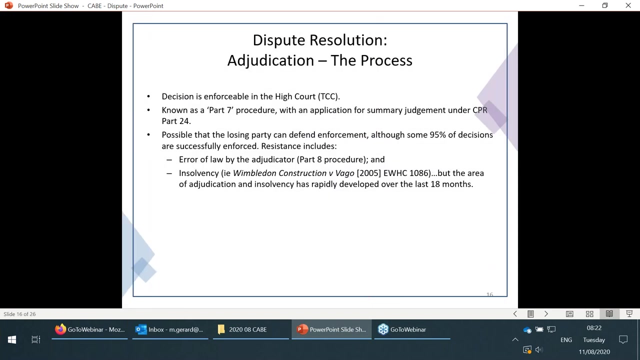 up to 14 days with just referring parties permission, or or, of course, both parties permission, or in excess of 14 days, with permission of both parties. usually, and from experience, most of our adjudications are between 28 and 42 days. the decision of an adjudicator is enforceable. 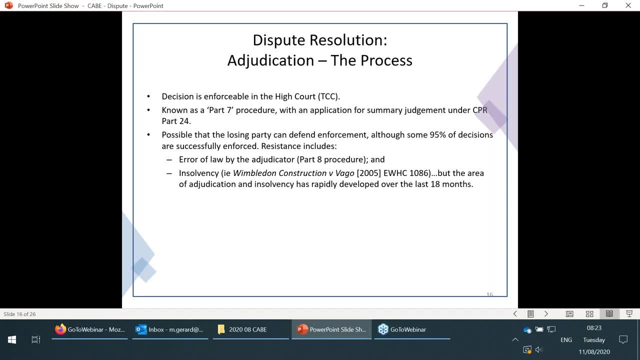 in the high court. this is known as a part seven procedure and it involves an application for summary judgments under the civil procedure rules, part 24.. it's possible the losing party can defend enforcement, although please take notes that 95 percent of all decisions are successfully enforced. 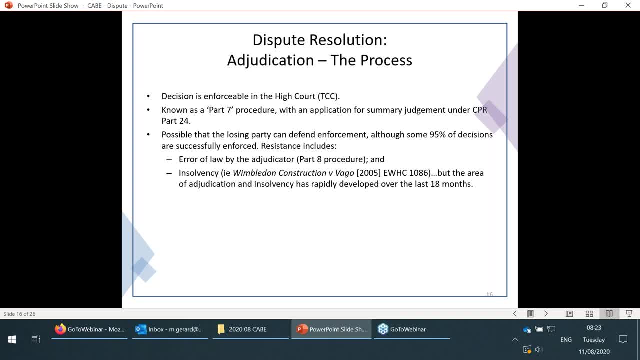 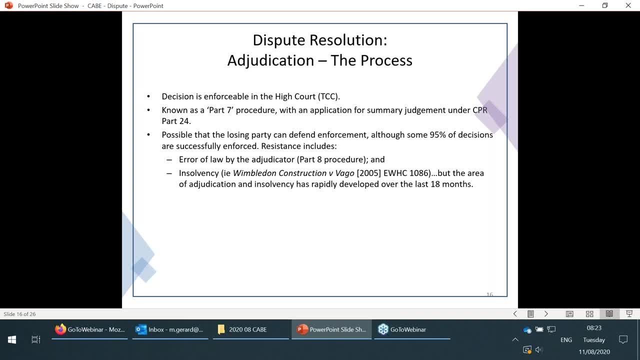 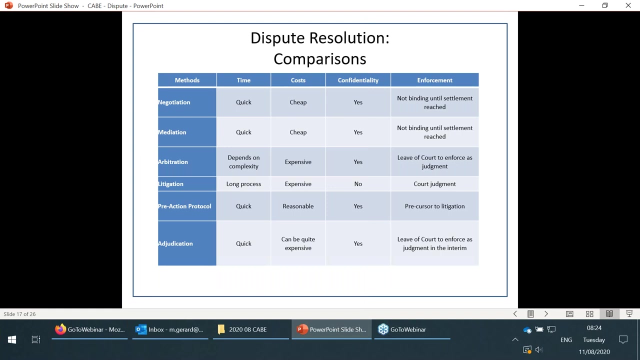 the great of a case. early income have unlaid'ed sellers to the court and feared that left for the correct the case as you work with your lenders to determine if you are going to have a received Нам lenity months. So where are we on dispute resolution and the methods? Well, the comparisons is that you can see that at the very top there, negotiation is very quick, as you might expect. 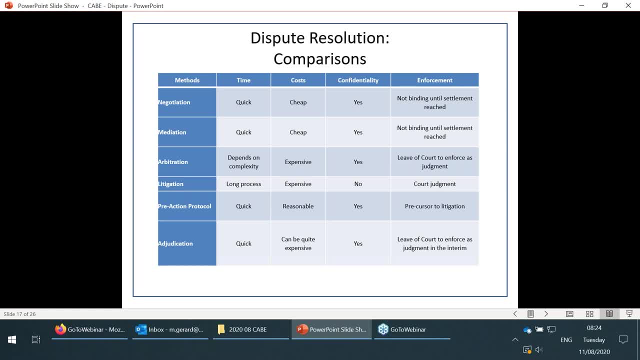 The cost is cheap because there are no outside parties involved. Confidentiality is guaranteed. However, on negotiation, is that nothing is binding until settlement has been reached. Mediation from experience is a very good form of dispute resolution. It is quick, It is relatively cheap. 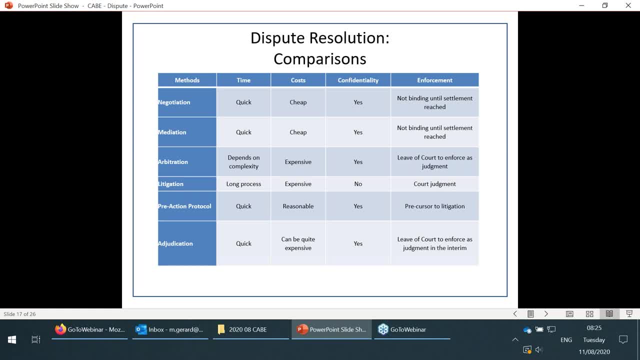 And, of course, again it is Confidential. and enforcement, again very similar to negotiation, is that it's not binding unless a settlement is reached and a settlement agreement is then executed- Arbitration- that time, in relation to arbitration, it can be quite long, It can be just as long as litigation, It can be expensive and it is expensive. 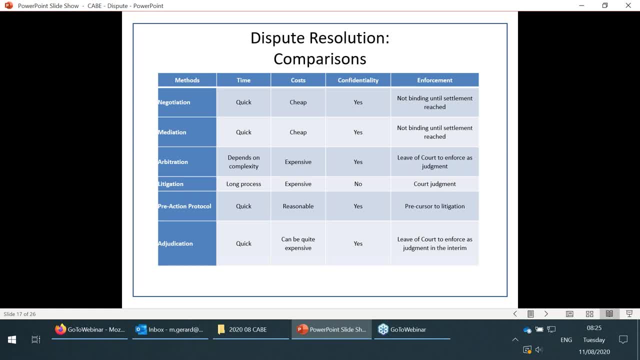 But the confidentiality Confidentiality is of course it contains two within the parties. It's not in the public arena unless, of course, one of the parties decides to run off to the court and challenge the arbitration decision or there's a jurisdictional issue. 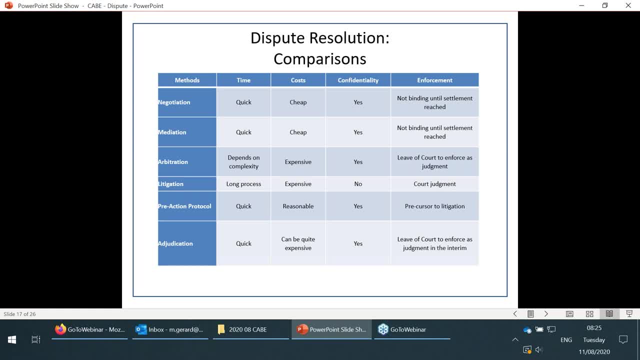 And in relation to enforcing judgments, you need leave of court to enforce that Litigation- that It can be quite a long process, even in the small claims and especially where we've got this pandemic is currently going on. The course can be slow, although the costs are, I've said, expensive. 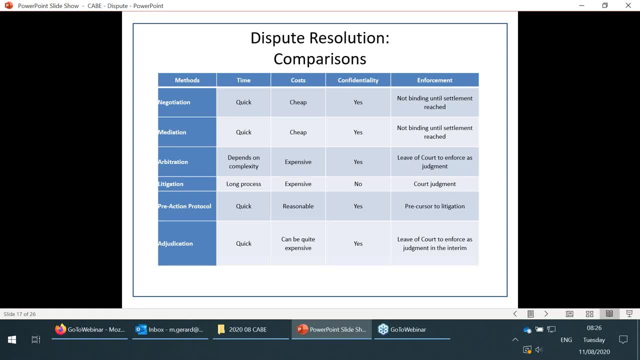 If you can DIY, and especially small claims, of course, when you're not involving lawyers, it is relatively inexpensive. In litigation there's no confidentiality, It's out there, It can be seen by the public And enforcement is by way of court judgments. 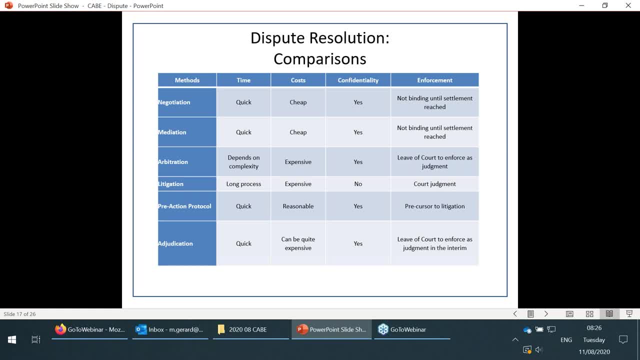 Creation protocol. that is very effective, It's very quick, The costs are quite reasonable And, again, confidentiality is guaranteed And once you actually reach an agreement in relation to having the action protocol, uh, meeting or mediation, you can. if it's uh, if this, if the dispute is settled, then 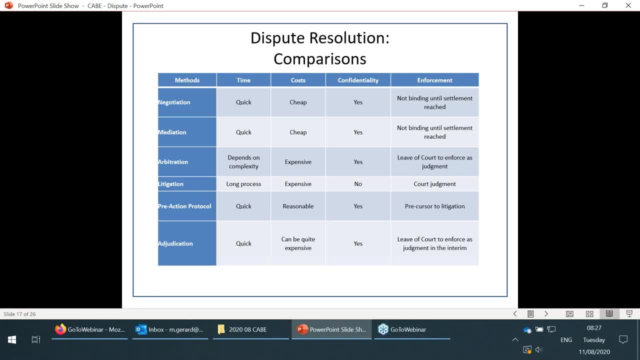 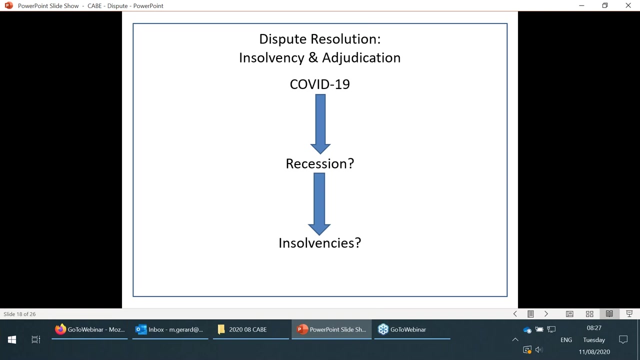 a settlement agreement isn't executed, an adjudication: it is quick, it can be expensive. um and uh again. confidentiality is guaranteed and you do have a court enforced decision right up to date. here we have is this pandemic um and um. i i prepared these slides um a few weeks. 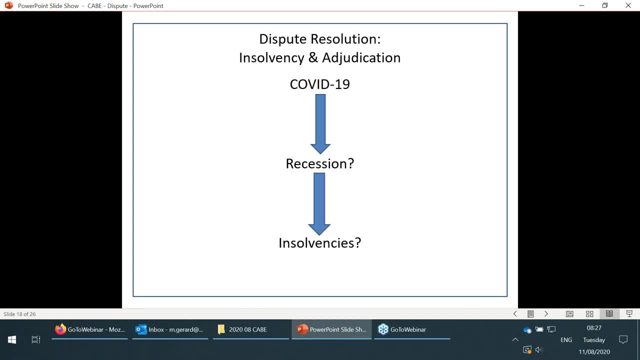 ago. um and um, i've said: there we've got covid 19 and everything's a serve in unparalleled, unprecedented times. um, and are we going into a recession? um, well, it does look as if it's a guarantee that we are going to recession and we're not going to recession and we're not going to. 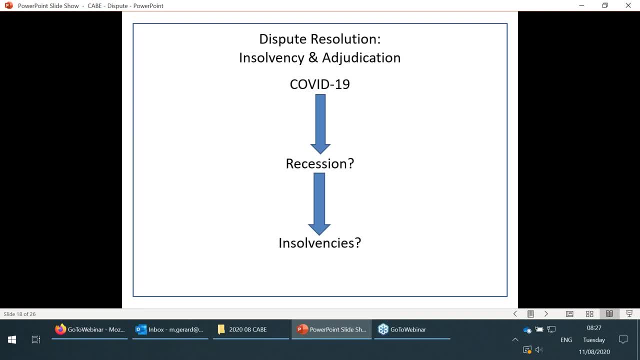 in fact, uh, it looks as if we are in recession- is the question is: how deep and how long and how damaging is this recession going to be? and, uh, one of the casualties, or one of the areas of growth- whichever way you like to actually look at it, uh- is insolvencies, um, which we've seen over the last. 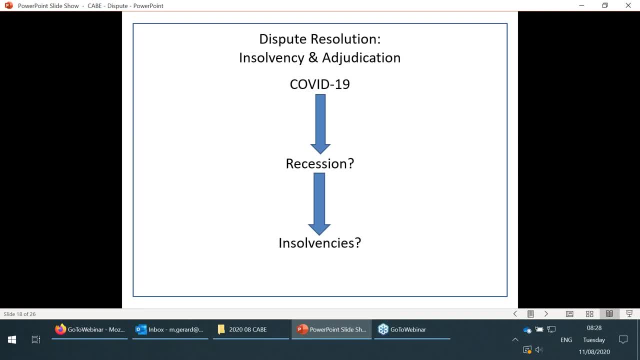 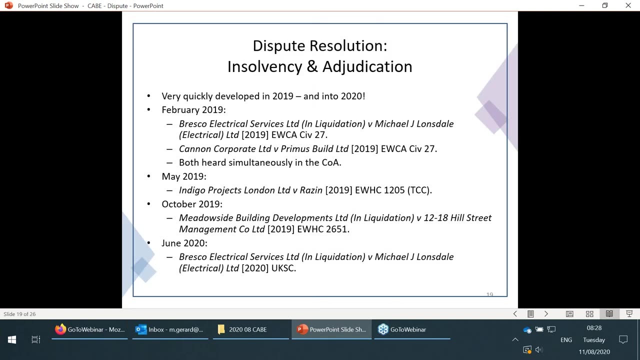 few weeks some major headlines on companies that are folding um and the construction industry and engineering industry industries uh are not going to get off uh lightly, so that brings us into insolvency uh, and adjudication, and i'm not going to go into any sort of detail uh in relation to 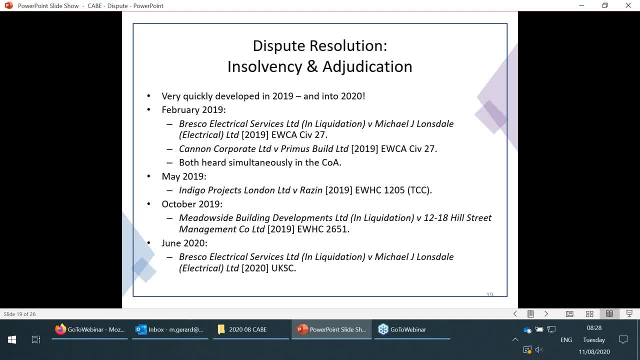 insolvency, because that is, uh, it is quite a complex area, um, it's a uh, it's now a growth area, unfortunately, um, but just to say that, uh, where we're now in august 2020, um is a very- is very different to where we were um 18 months ago, 24 months ago. it has developed, uh, very very. 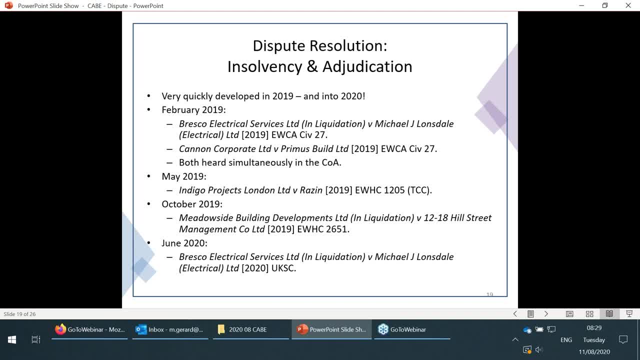 quickly, um, whereas if a company was, uh was insolvent um then, uh, two years ago, then it was virtually pointless and actually, um, i've of course bring proceedings against but that insolvent company, the liquidators, to actually uh bring any proceedings uh in adjudication because, uh, quite 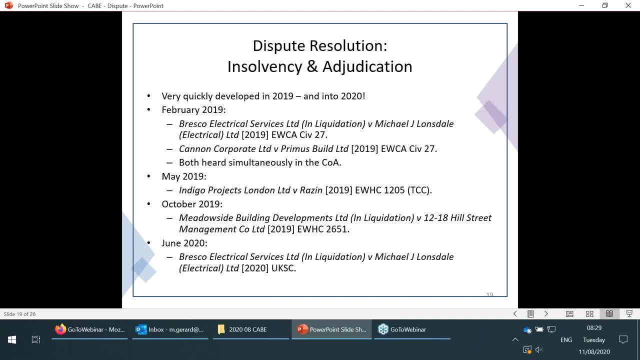 simply, the adjudication is not going to be able to bring any proceedings uh in adjudication decision would not uh will not be enforced. well, as i said, that's been changed by various um uh by various cases over the last 18 months. uh, we've got the uh the briscoe um electrical services. 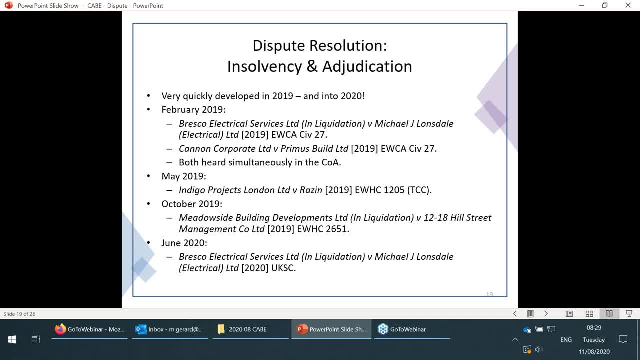 versus uh lonsdale uh. in fact, that started off uh at the tcc february 2019 and that has now gone all the way uh to the supreme court uh in june um 2020. um the uh we have the meadowside building. 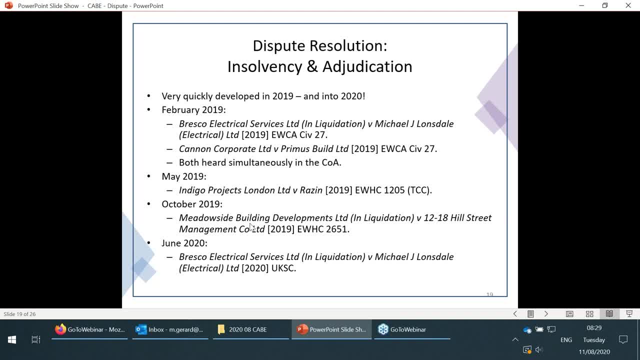 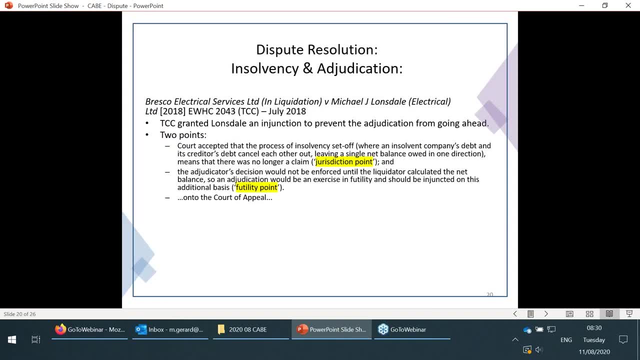 developments uh happening on in october 2019 at the high court um, and also the indigo projects versus uh razor. but very quickly uh, i'm going to uh go over the briscoe uh and lonsdale. and there was two points that came out uh of the of the initial court case, um, and that was a jurisdictional. 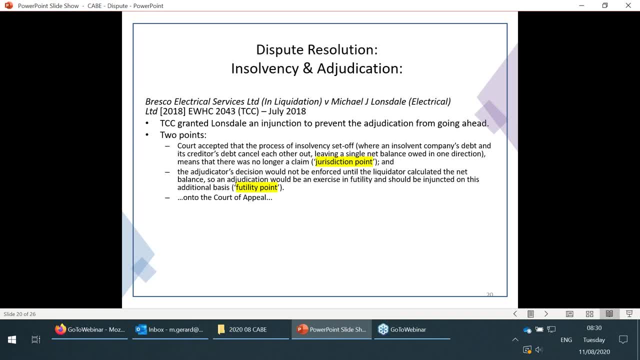 point and the point on utility. now the court accepted, the process of insolvency set off. uh, and this is where an insolvent company's debt, um, and it's in and it's creditors debts cancel each other out. leaving a single net balance in one direction means there's no longer a 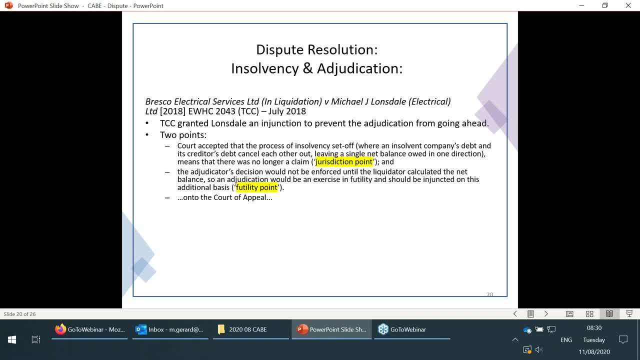 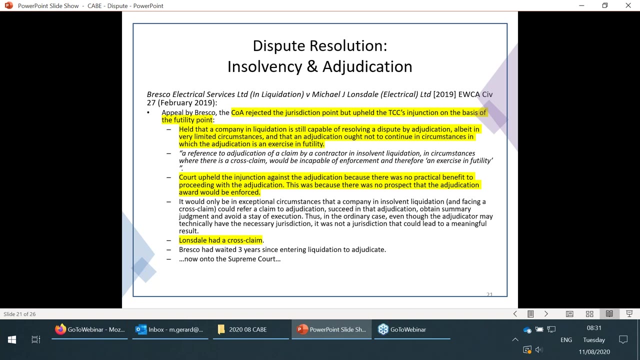 claim. that was a jurisdictional point and the futility point was that the adjudicators decision would not be enforced in any event until the liquidator had calculated the net balance. so they failed on the on the uh futility points at the tcc. it was then appealed um and um, the um uh and basically on the uh. on the. 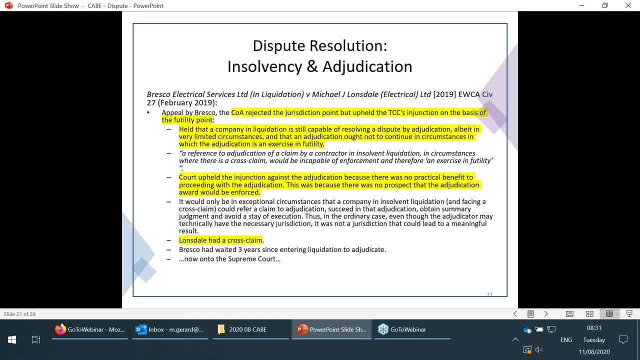 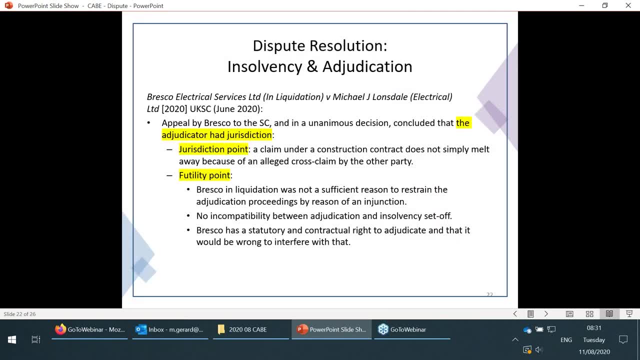 course of appeal, um, the uh, the courts uh agreed with the, the court of first instance and then that went all the way to the supreme court. that was only in in june. and the uh in relation to the supreme court on the futility points was that briscoe, who is in liquidation, was not a sufficient reason to restrain the adjudication. 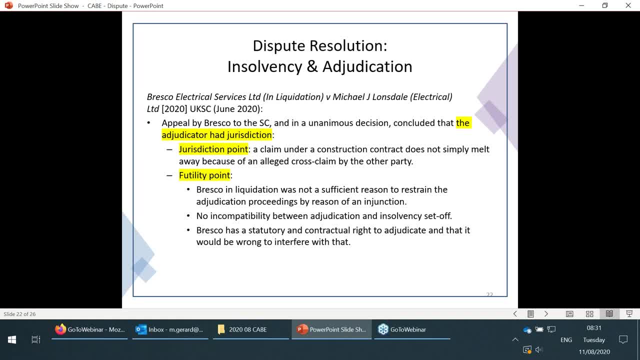 proceedings by reason of the injunction, and the court held that briscoe had a saturated contractual rights to adjudicate and that it would be wrong to interfere with that. of course there is still the question: would it be enforced? but uh, we're gonna, we're gonna wait and see on. 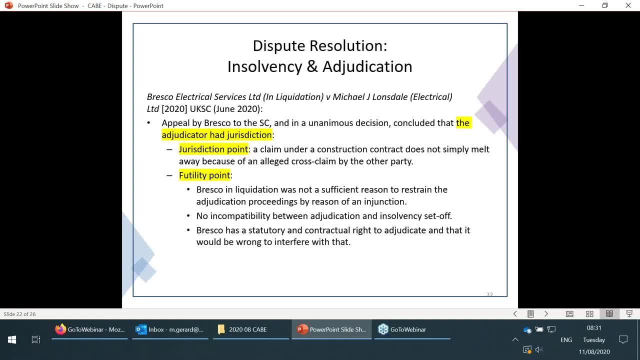 that. but let's say adjudication, uh, uh, adjudication is not going to be enforced, but, uh, we're going to be asking to know what the, the, the cost of the along way, um and um, it's, um and it's come a long way in a very short 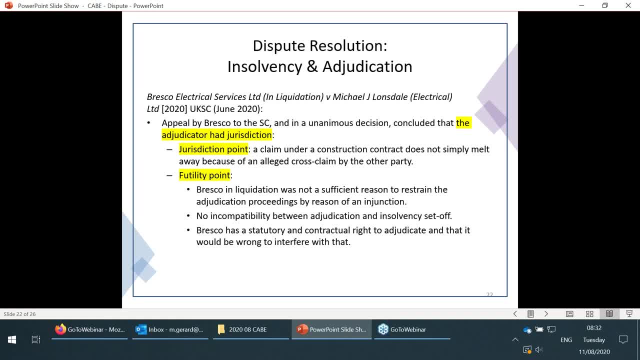 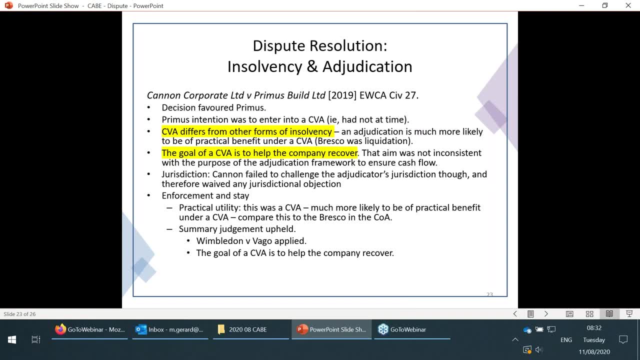 space of time and there's going to be, i believe, quite a few um cases in the future involving insolvent companies. um, because if we take the, the another case can incorporate versus farmers builds. this involved a cva, um and um, And what the court said in relation to the CVA was that the CVA was different to a company. 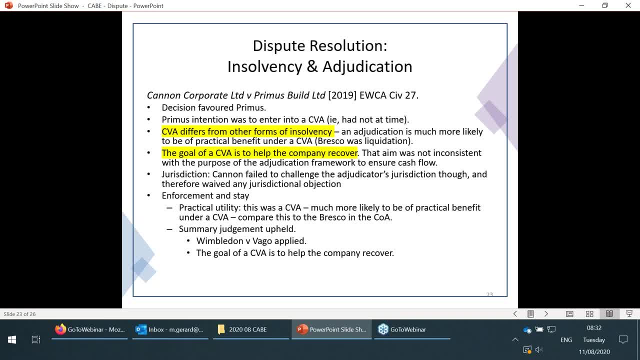 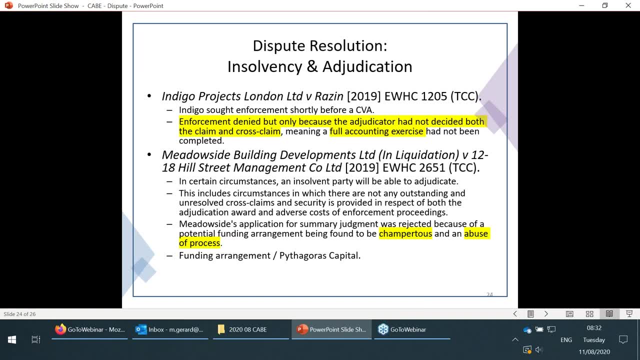 that was in liquidation, because the goal of the CVA is to help the company recover. And on Indigo Projects Limited versus Raisin, this was a TCC decision. the enforcement was denied only because the adjudicator had not decided both the claim and the cross claim. 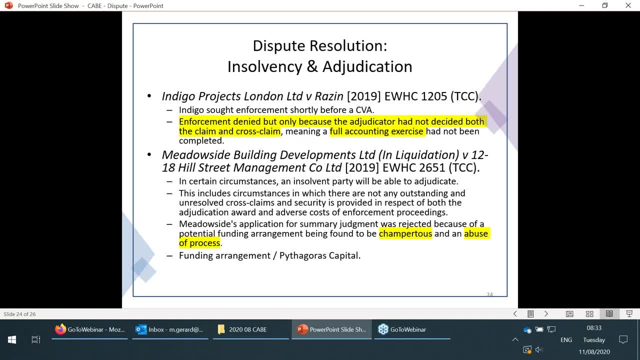 meaning that forecounting exercise had not been completed. And in Meadowside Building Developments versus 18 Hill Street Management, the reason why the Meadowside application for summary judgment was rejected- because it wasn't because of Meadowside's liquidation But because of it- was found. the judge found that the arrangements in relation to the funding 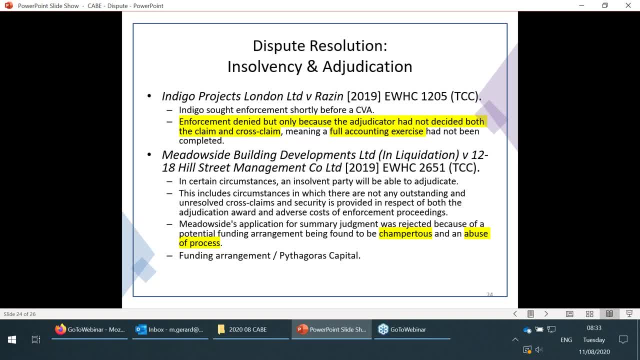 to be champetos- it's easy for some people to actually say that- and also an abuse of process. Now I believe that is going is due for an appeal sometime, But again, I don't think we've actually heard the last of that. 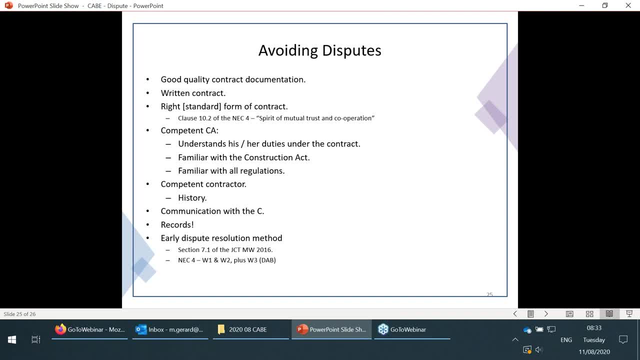 Let's get on to avoiding actual disputes. We must have good quality contracts documentation. You must have a written contracts- absolutely crucial. There must be the right standard form of contract. You must have ensured that is a competent CA stroke, A competence engineer refirus. 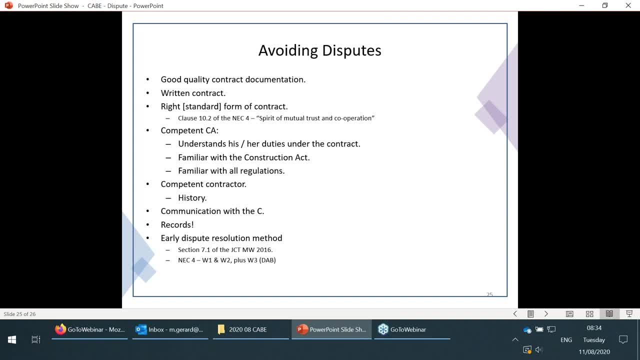 That sort of kind of thing, Yes, under the NEC, and that person understands his or her duties under the contract, is familiar with the construction acts and is familiar with all the regulations. also, there must be the contractor stroke. the subcontractors must be competent, and there and there must be. 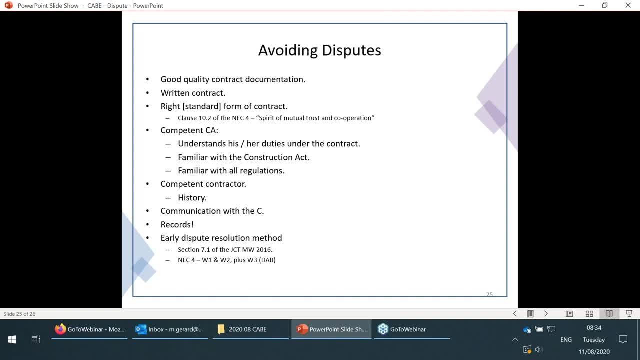 history with those contractors and subcontractors. there must be communication at all times with a contractor. the most important thing of all is records. records records early dispute resolution methods, as I said before, comes out of our contains in the various standard forms of contracts, including the JCT suite of contracts. 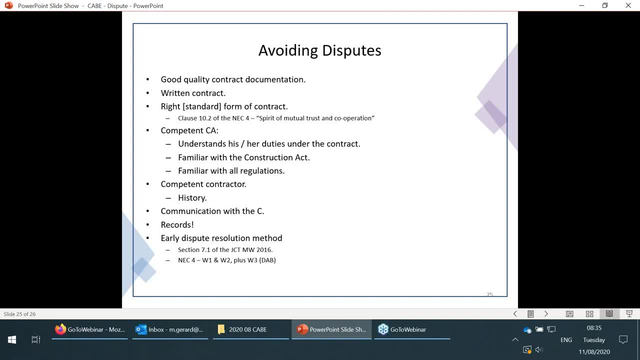 and also the NEC, for which option w1 and w2, that is for the senior reps. w2- momentous rights- is where the- where adjudication is the prize- are able to actually adjudicate. w1 is where the parties can adjudicate under that because the sort of works ratio carrying out 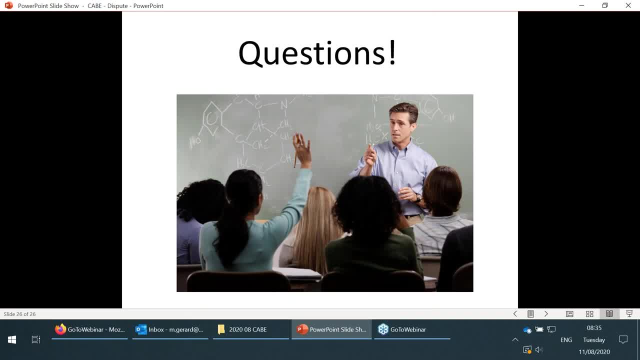 and questions. thank you for listening to me. thank you, Michael. thank you. so, in terms of questions, we haven't really had any come in as yet. so if people have any and they want to send them through now, they can, and I'll just mention a couple of things from HQ while they do that. 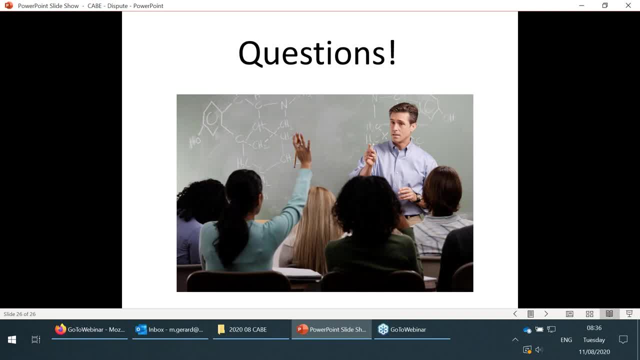 so hopefully you will see it by now, but Cape have relaunched a newly structured certificate and building control course, along with a fire safety practitioner certificate. so the fire safety course contains the essential learning for those working in the design, construction and inspection areas of fire safety and 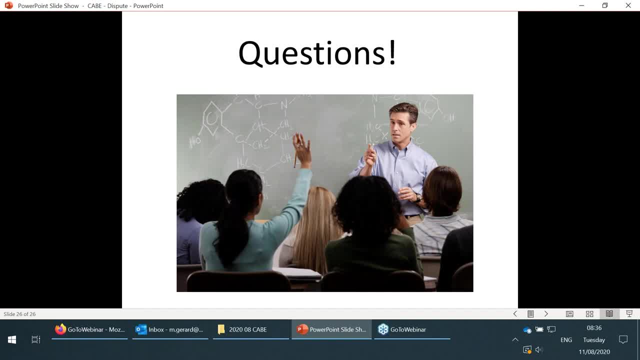 it provides a basic understanding of how to interpret and apply in a practical way way Part B of the Building Regulations. It touches on relevant British standards and approved guidance including BS 9999,, BS 9991 and PASS 79. Hopefully that sounds of interest. 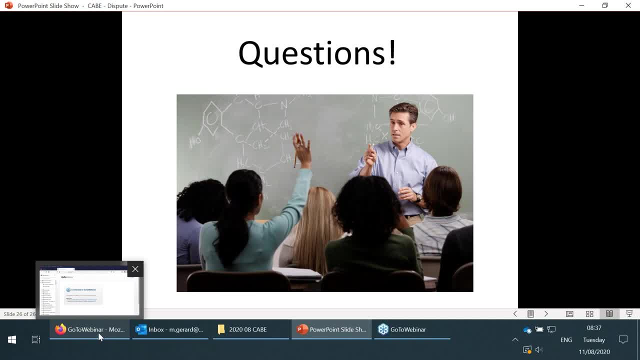 to some of you. All of the information is on our website, so please do go and have a look. We have our usual Webinar Wednesday scheduled for tomorrow, which is Active Buildings in Practice, So hopefully I'll see some of you online tomorrow as well. So let me just 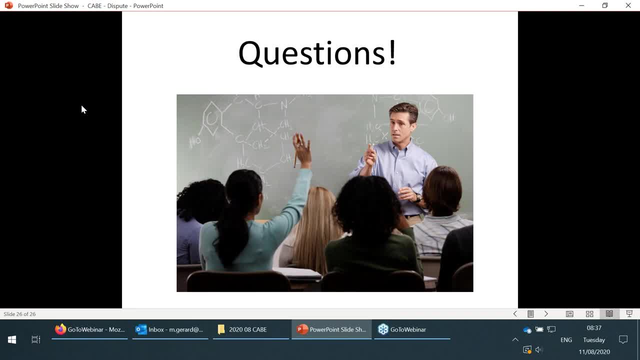 have a quick look. We've got a question coming in asking what the best contract is to use for building. Right, Okay, It's impossible to actually, I'm afraid it's impossible to actually answer that question just with that level of information, because if you gravitate, for example, towards the 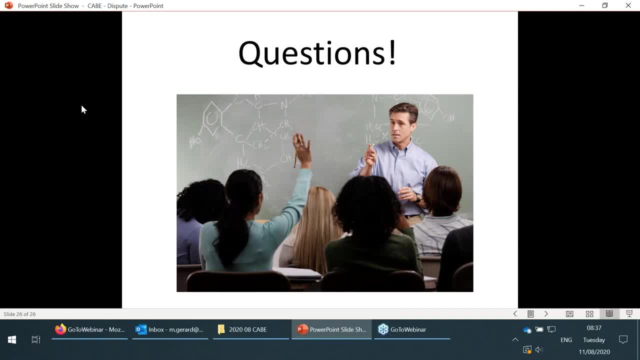 JCT Suites. you have several different editions of JCT, So is there a design element involved? Is it a design and build? How large is a project? How complex is the project? If you're looking at a project that's 50 million, it's going to require different procurement routes to a contract, So that's. 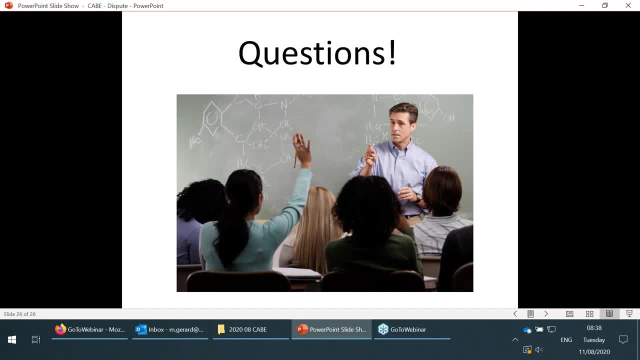 only priced at £250,000. So £250,000 might only require a JCT- minor works, whereas the £50 million is going to require the standard form of building contracts. You've also got, of course, the intersection of the design for the project, the JCT and the JCT course. 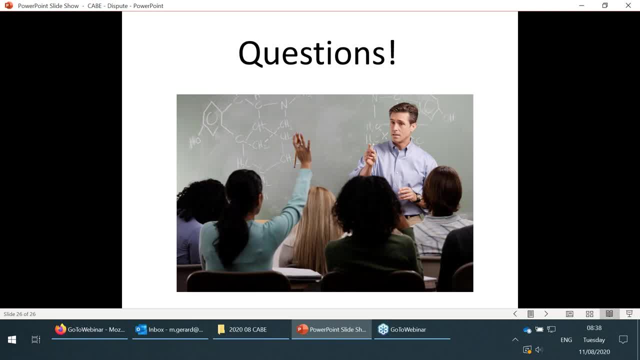 there as well, and so on. So it's a significant requirement of the JCT. That's exactly right, And what needs to be done is to actually sit down to see, to work out exactly what that contracts actually is, what it's worth, what you want. 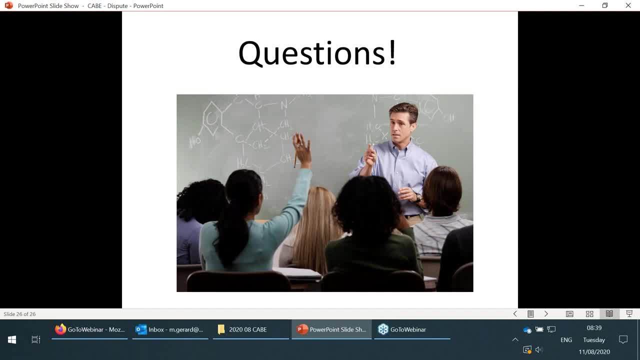 out of the contracts. Yeah, Yeah, um that uh, you actually that the uh the employer strike the professional team? um actually wants, for example, um is the uh, is everything going to be handed over to the contractor, who's going to be responsible for all of the uh employment of all the special subcontractors, or is there um some? 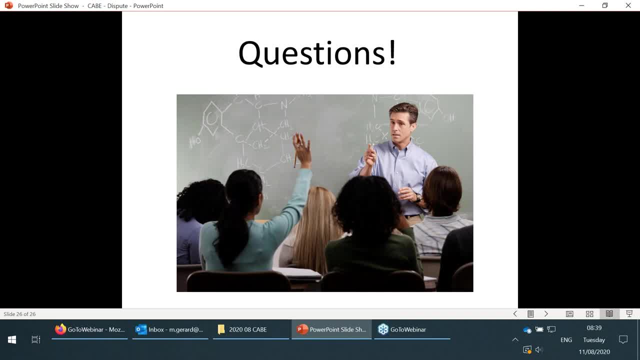 control, uh, that the employer wishes to have in relation to the selection of some of the subcontractors, um, or even um directs, uh, some of the directs or subcontracts. so, um, it's, uh, i'm not, i can't answer that question directly, but um, you do need to actually uh sit down and see exactly. 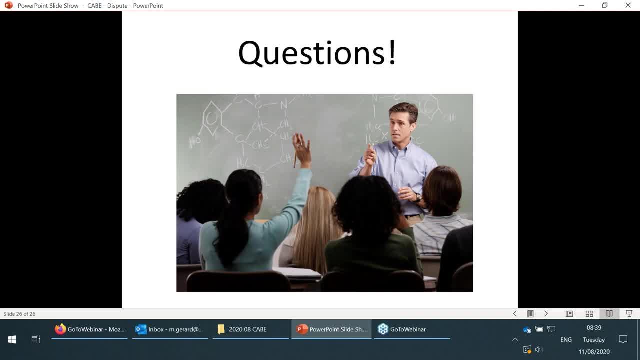 what's involved in that project and then look at the uh, the actual contracts uh, to see which one best fits that particular uh project. okay, thank you. um, so we've had a gentleman ask whether there are any differences between scotland and england in terms of dispute. 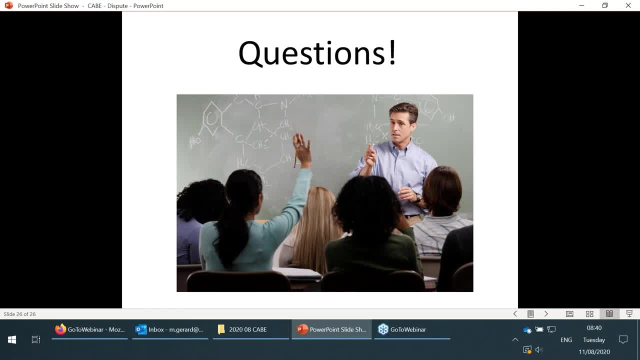 resolution: uh, very good question. um i must admit um i don't uh travel well uh past, uh past the border um, but um, so my practice area is exclusively uh within um england um, but um i that there are differences, yes, there are, um they have. they do have um a form of the construction actor, i believe uh um up in scotland um again, i've never 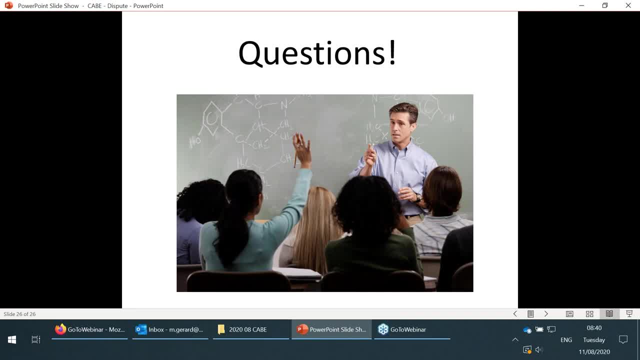 had um a uh. i've never ventured into the scottish jurisdiction um, but they do have different uh methods um, different regulations um and different forms of um of disparate resolution, although most of it uh is based on england. okay, we've got another one asking whether the pre-action protocol meeting is compulsory and who. 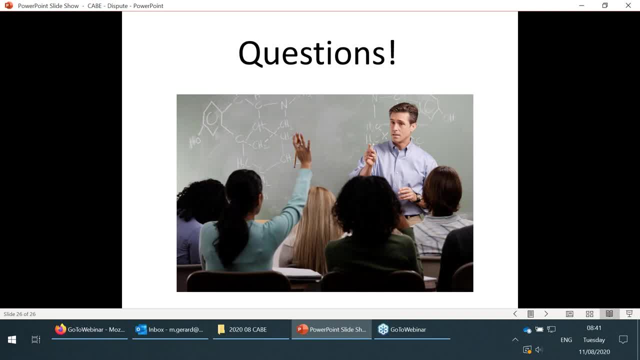 attends? uh, very good question. uh the pressure, uh the pressure protocol, um, it is all but mandatory, and i'll say all but mandatory, um, it doesn't prevent a party, a claiming party uh for running off and uh filing and serving um a claim for um, but uh, why, besides, uh, those parties that ignore? 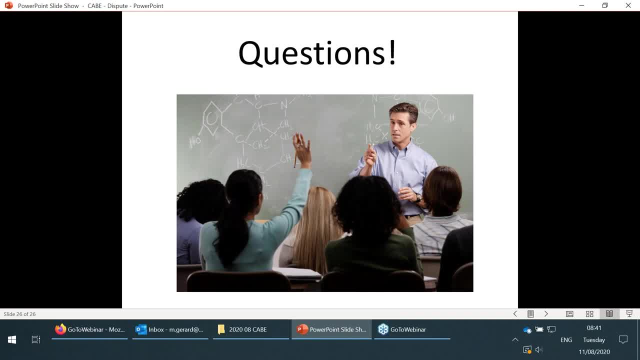 the pre-action protocol because, uh, they do run the very real risk um of having an adverse cost order um, even if they are successful uh at the uh all the way to a hearing. so, first of all, it is absolutely crucial um that the pre-action protocol um is, um is is instigated um that there are um some that there will be one or two um. 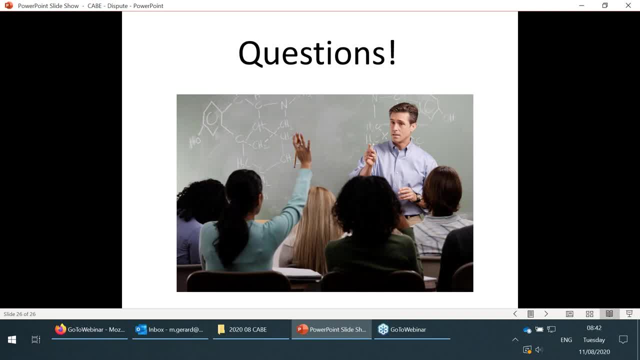 instances where um the uh, by ignoring the pressure protocol, um it is, um, um is is commons allowable, uh, for example, uh, if the dispute is getting very close or the matches get very close to the limitation act, um, but uh, in relation to mandatory, and you know. but in relation to mandatory, and you know when it comes to mandatory, and you know when it comes to. 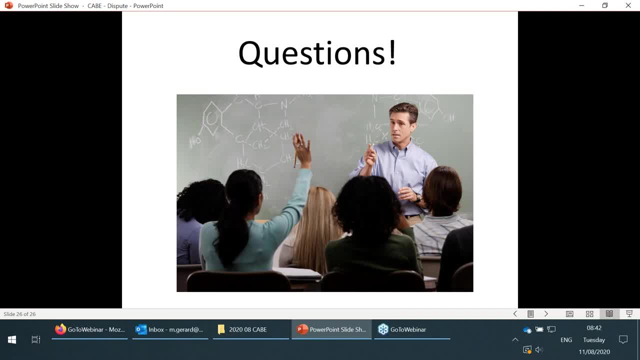 whether or not a meeting is mandatory. it's not mandatory, but it's um, uh, it's a very, very good idea, uh, to make sure you do go through the pre-action protocol because, as i said, um, it is. it is so crucial when, if the, if, the, if the matter is going to run all the way, um, into court, into a. 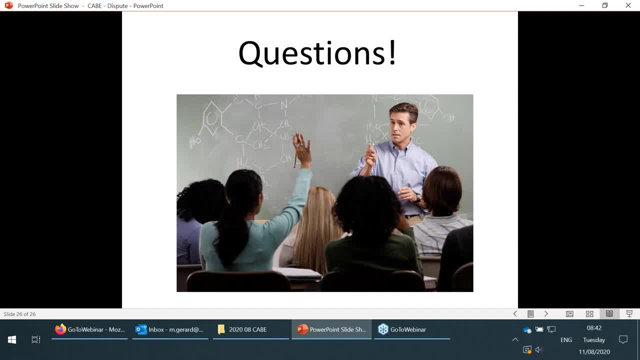 hearing. you need to demonstrate uh, that uh. you know that that you um, as one of the parties, attempted to actually um, uh, to actually um, meet with the other side of the very early on and attempt to um, to actually resolve the case without going off and spending 10, sometimes hundreds of thousands. 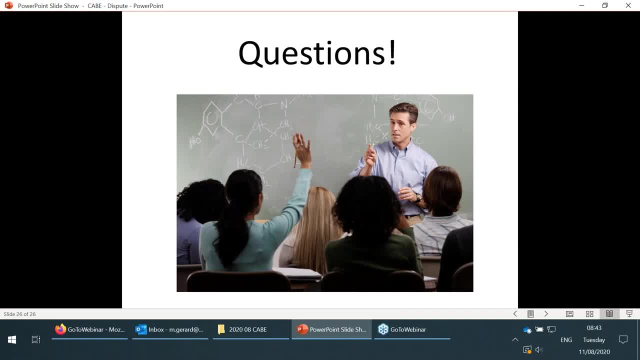 of pounds on legal costs and experts? uh costs? uh, in relation to the meeting? um, there is no. uh, it's not mandatory to have, say, for example, mediation once there's an exchange of the uh of the letters, ie the letter of claim and then the response, that letter of claim- uh, there is no. 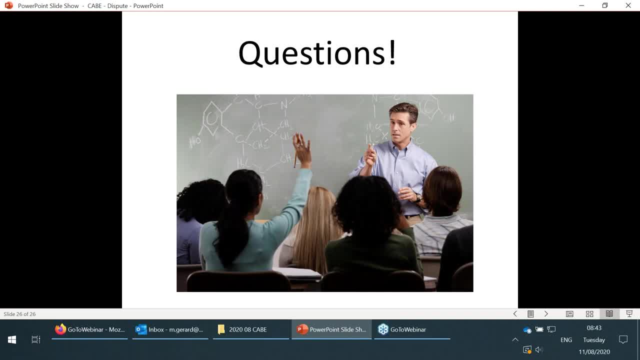 there's no requirement to actually have a mediation, but, uh, the parties, um, should then have a meeting that could be around a table, um, uh, just the parties, on a one-to-one basis. they could have the lawyers there in attendance, um and um. but but again, um, it is. it is crucial that um, uh, there is a.